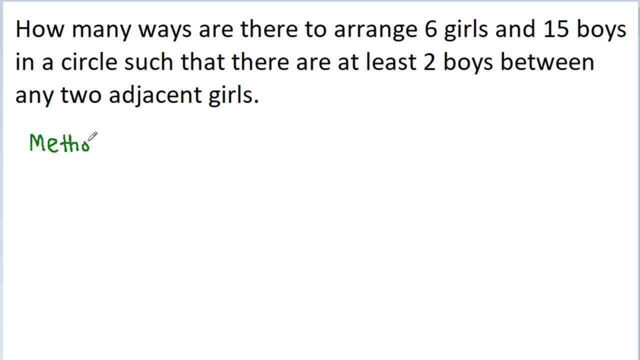 So the first method, method 1, is: let's draw what is going on. So we have a circle and we have 6 guns and 15 boys. So first arrange these 6 guns, So 1,, 2,, 3,, 4,, 5,, 6,, 7,, 8,, 9,. 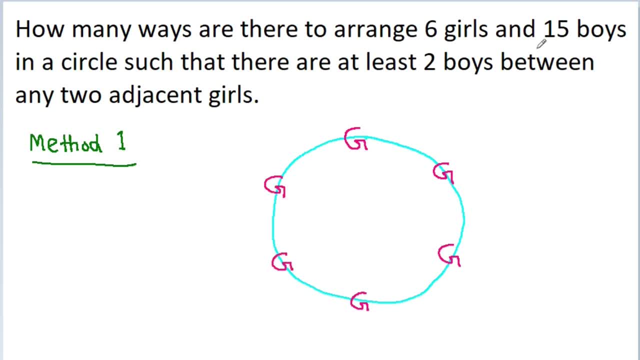 10,, 11,, 12,, 13,, 14,, 15,, 16,, 17,, 18,, 19,, 20,, 21,, 22 and 23.. I will write the third position: 5,, 3,, 4,, 5,, 6,, 7,, 8,, 9,, 10,, 21,, 22, 23.. 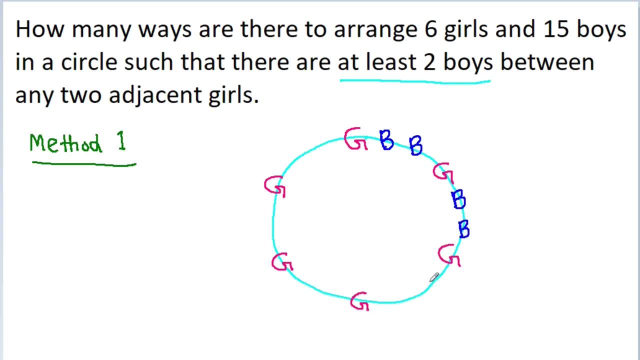 And we are told that each of these 2 guns has at least 2 boys. So we have these two boys of 3 positions. So for each of these 2 guys, put exactly 2 boys between 2 adjacent guns. That is why these two guys will be bigger than each other. So in this way you can. 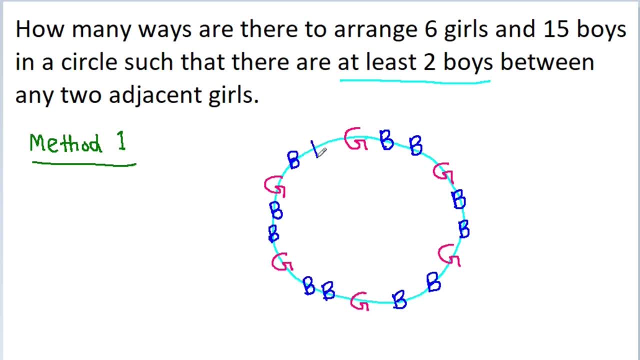 1 and 2,, 1 and 2.. Now the condition is satisfied And we have arranged total 2 and 5 boys. So we have 3 boys left. So we can arrange those 3 boys anywhere in the circle 1,, 2,, 3.. We 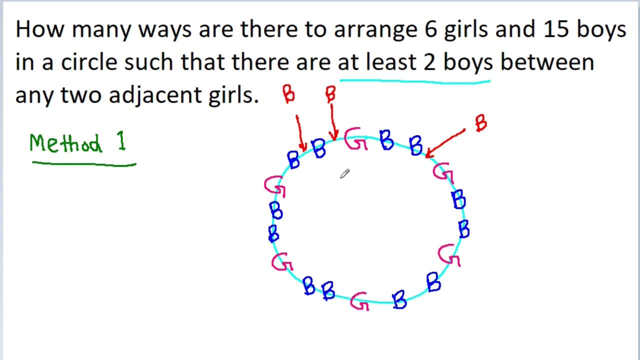 can arrange it anywhere in the circle. Now we have to think about the number of ways we can make the arrangement like this. So what I am going to do is I am taking 1 girl and 2 adjacent boy and making them a group. So this is the first group, This is the second. 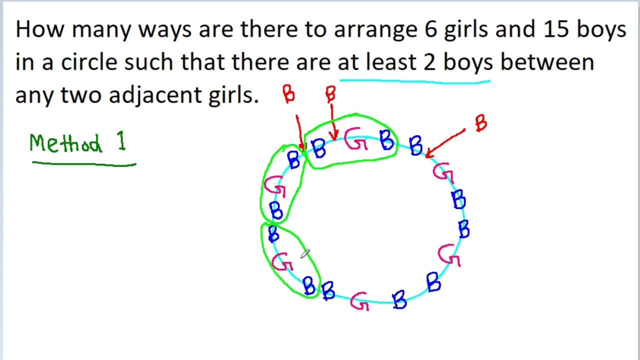 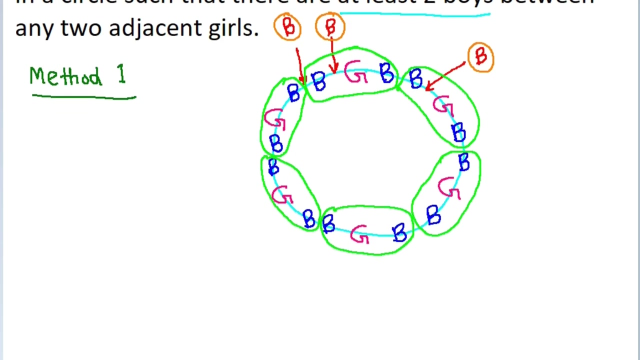 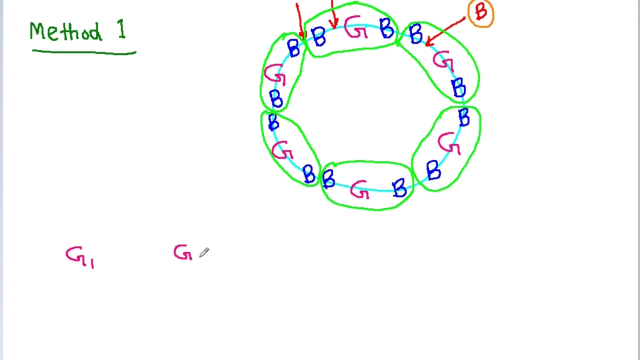 group. This is the third group And it is the fourth one group and fifth group and sixth group. so can I say that we have to arrange these six groups and these three boys in a circle. so here we have six girls: g1, g2, g3. 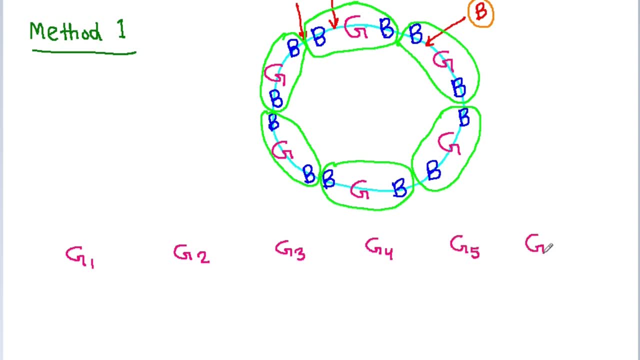 g4, g5 and g6 and to make group. for g1 we have to select two boys out of 15 boys. so we can select two boys out of 15 boys in 15 c2 ways and these two boys can be arranged in 2 factorial ways. and now for g2. 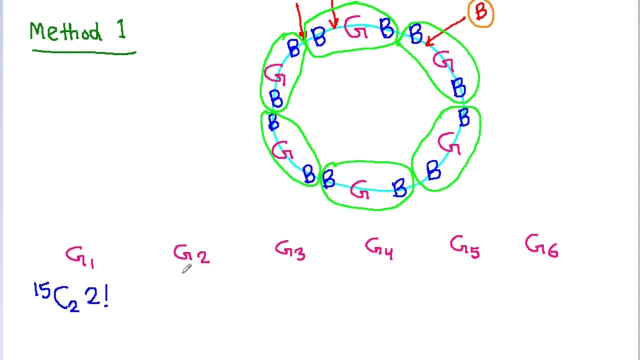 we have to make group out of 15 boys of g4, give 1 half of the Forshak boys, so only 13 boys left. We have already selected two boys out of 15 boys. So here we have 13 boys left and we have to select two boys. and these two boys can also be arranged in two factorial ways. 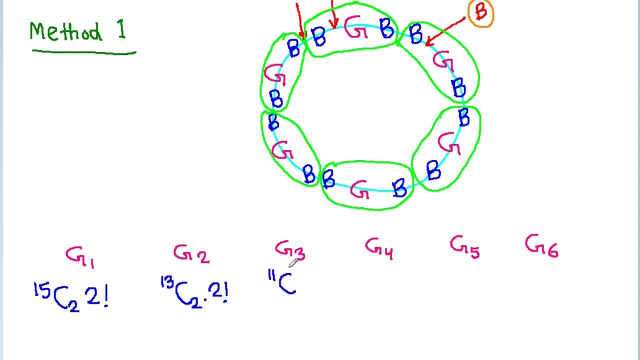 And now for G3. we have 11 boys left and we have to select two boys, and two boys can also be arranged in two factorial ways, and similarly for G4 it will be 9C2 into two factorial and for G5 it will be: 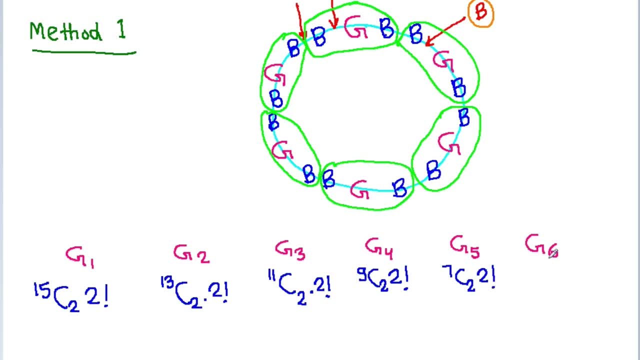 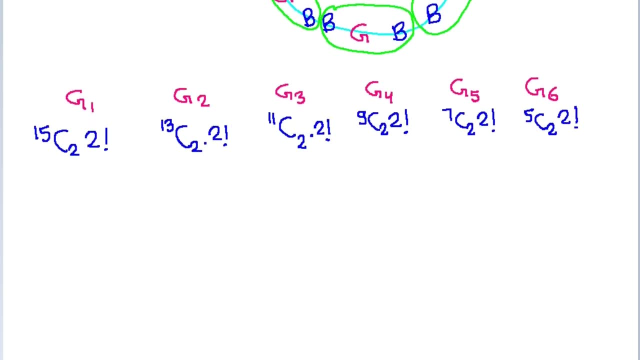 7C2 into two factorial and for G6 it will be 5C2 into two factorial. and now we have formed the six groups: B- G1, B, B G1, B- G2, B, B G3, B. 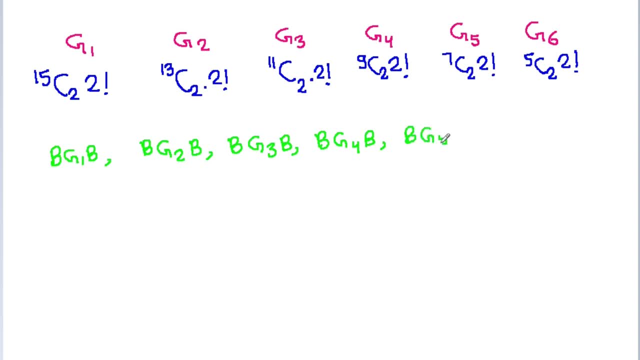 B, G4, B, B, G5, B And B, G6, B, And we have also three extra boys, B, B, B, So we have total nine objects. So we can arrange these nine objects in a circle by eight factorial ways, because the number of ways to arrange 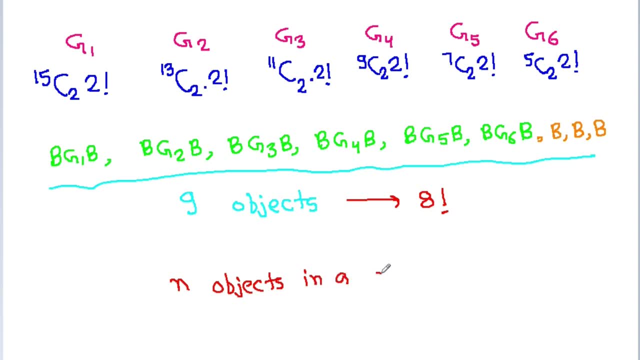 n objects in a circle is actually n minus one factorial, not n factorial. so here the total number of ways will be the number of ways we can form these six groups into the number of ways we can arrange these six groups and these three boys, that is eight factorial. so it will be 15C2 into two. 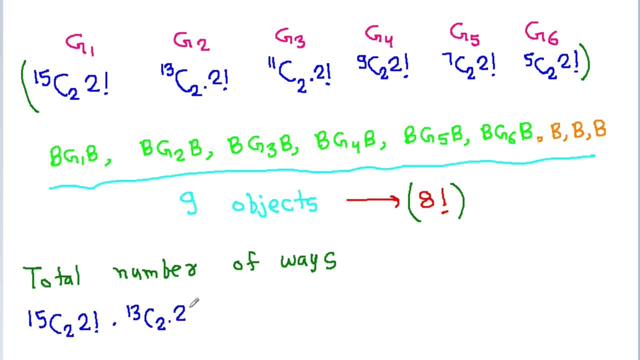 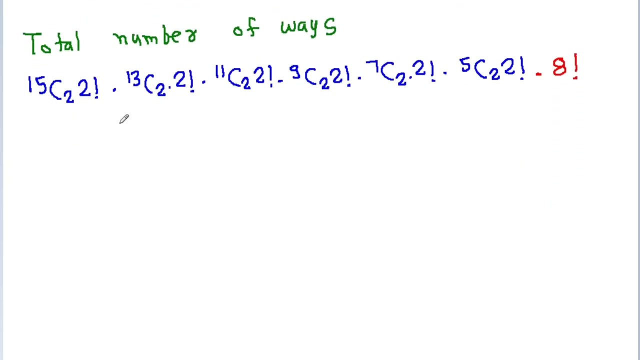 into 13c2, into 2, into 11c2, into 2, into 9c2, into 2, into 7c2, into 2, into 5c2, into 2 and into 8, so we will get 15c2 will. 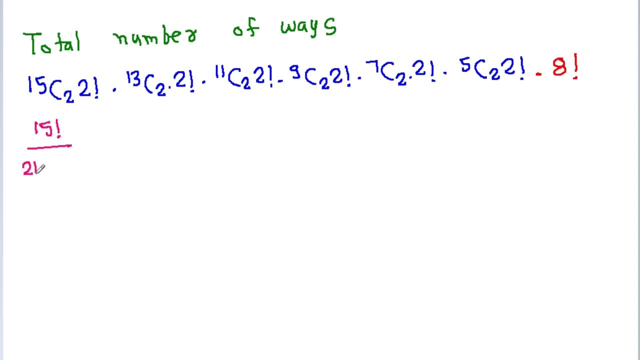 be 15 factorial by 2 factorial into 13 factorial. and we have 2 factorial into 13 factorial by 2 factorial into 11 factorial into 2 factorial into 11 factorial by 2 factorial into 9 factorial into 2 factorial into 9 factorial by 2 factorial into 7 factorial into 2 factorial into 7 factorial. 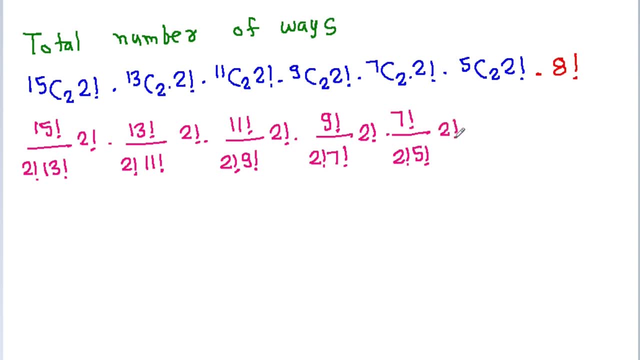 by two factorial into five factorial, into two factorial, into five factorial, by two factorial into three factorial, into two factorial and into eight factorial. and now these two factorial and two factorial get concerned, and similarly, these two factorial, these two factorial and these two factorians, these two factorians and these two factorians get concerned, And also these 13. 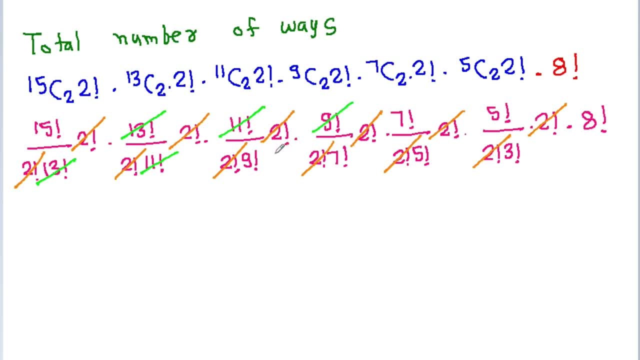 factorians, these 11 factorians, these 9 factorians, these 7 factorians, these 5 factorians also get concerned. So we get this 15 factorian into 8 factorian. by 3 factorian We get 15. 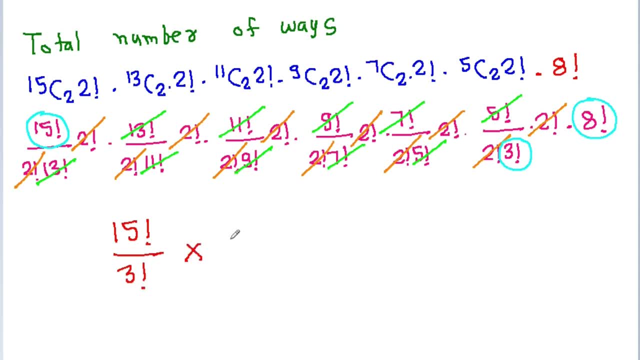 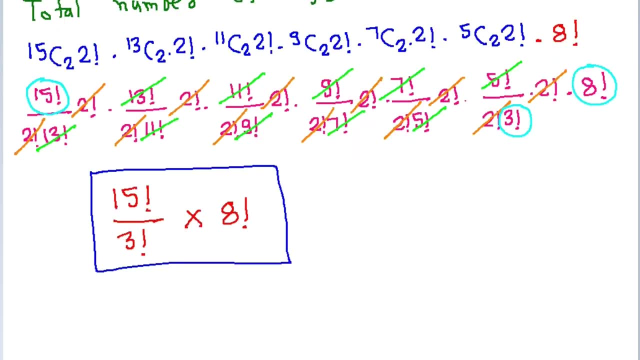 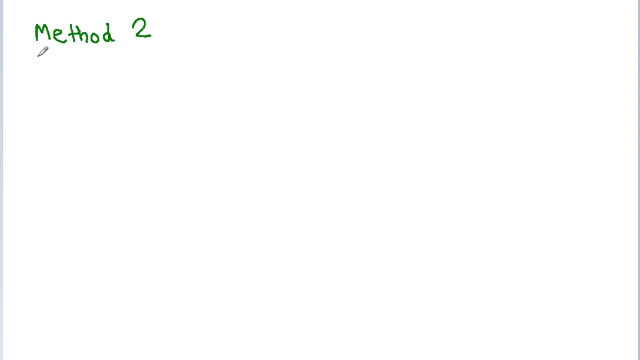 factorian by 3 factorian into 8 factorian. It is the answer. and now the second method, method 2, is here. we have a circle and we have 6 guns, So I am going to arrange these 6 guns in this circle. 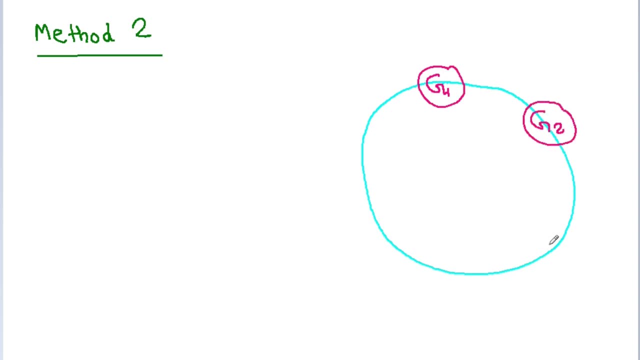 G1, G2, G3, G4, G5 and G6.. So can I say that the number of ways to arrange these 6 guns in a circle is 5 factorian. And now we don't know the number of boys between these guns, So I am assuming. 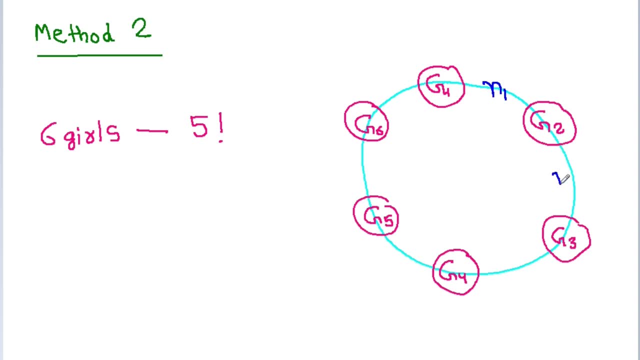 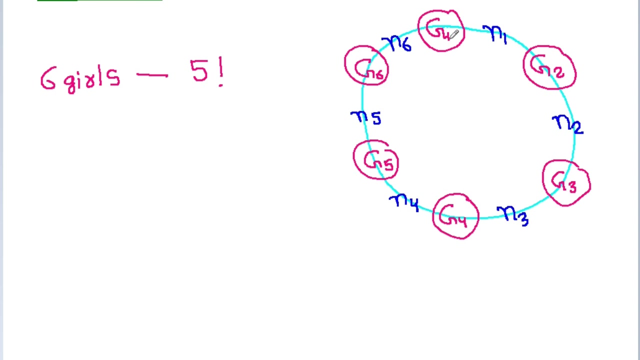 N1 boys between G1 and G2 and N2 boys between G2 and G3. And similarly, here n3 voyage, here n4, here n5 and here n6 voyage. So here can I say that n1 plus n2 plus n3 plus n4 plus n5 plus n6 is equal to 15, because 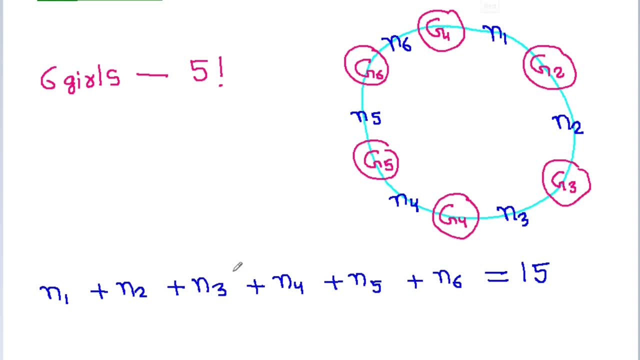 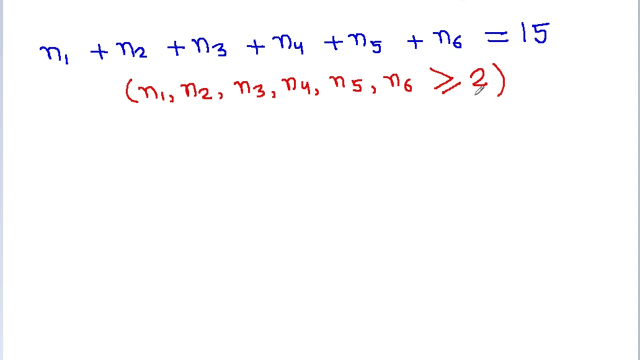 we have total 15 voyages. and there is a condition also, that is n1,, n2, n3, n4, n5 and n6- all should be greater than or equal to 2.. And now here, n1 is greater than or equal to 2.. 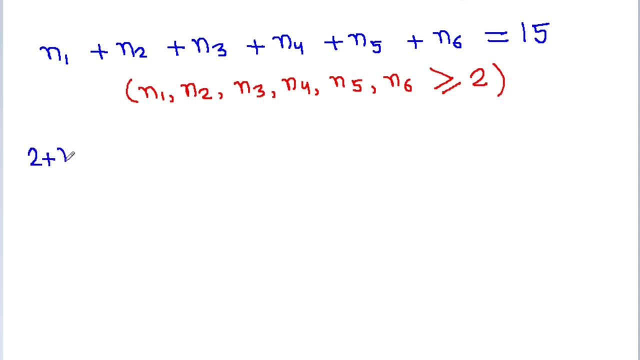 So we can write n1 as 2 minus sum n1 dash, n1 plus n2 plus n3 plus n5 plus n6 plus n6 dash. and similarly n2 can be written as 2 minus n2 dash. n3 can be written as 2 minus. 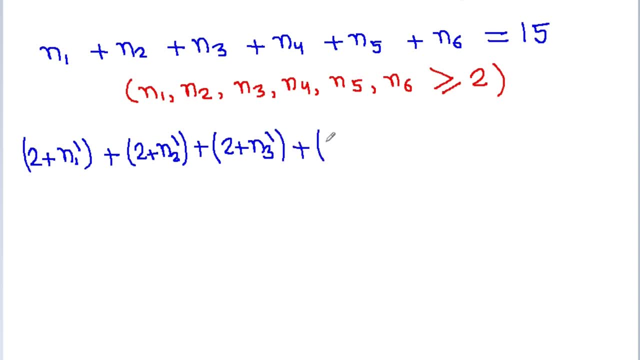 n3 dash and similarly n4 will be 2 minus n4 dash and n5 will be 2 minus n5 dash and n6 will be 2 minus n6. dash is equal to 15.. And where n1 dash is equal to 15.. 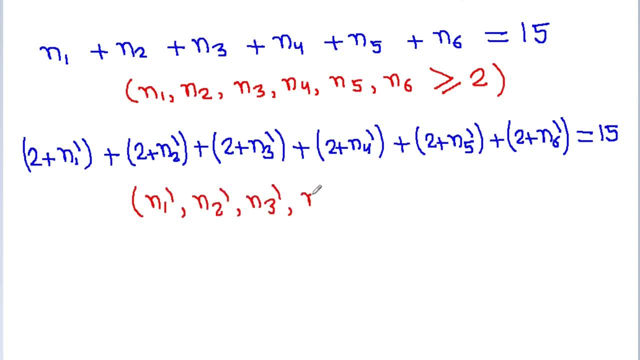 n2 dash, n3 dash, n4 dash, n5 dash and n6 dash is greater than or equal to zero. So we get n1 dash plus n2 dash plus n3 dash plus n4 dash plus n5 dash plus n6 dash is: